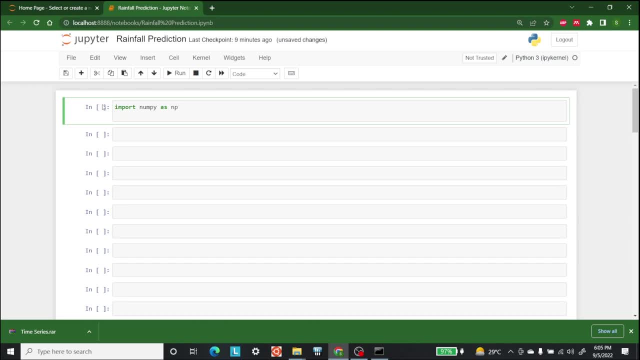 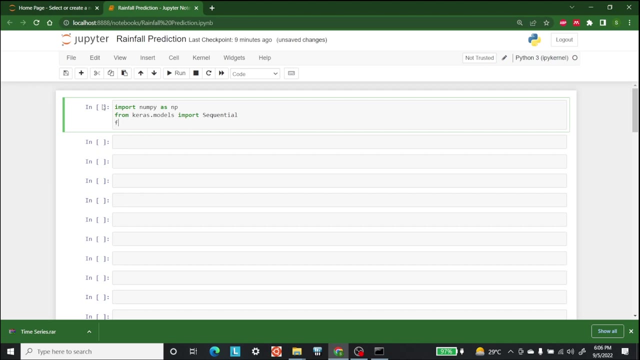 is numpy, So write import numpy as np. After that we need to have a few Keras models, So let's write from kerasmodels import sequential. After that, import a few layers So they are available in keraslayers, So let's import. 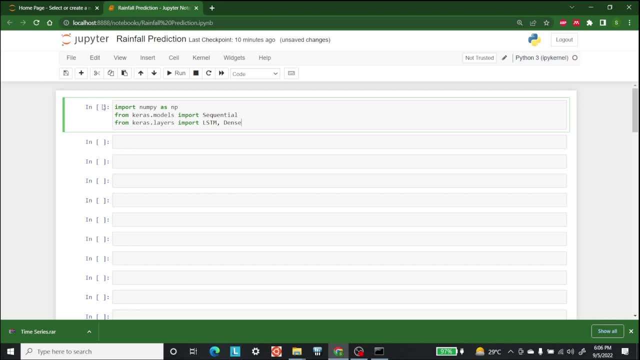 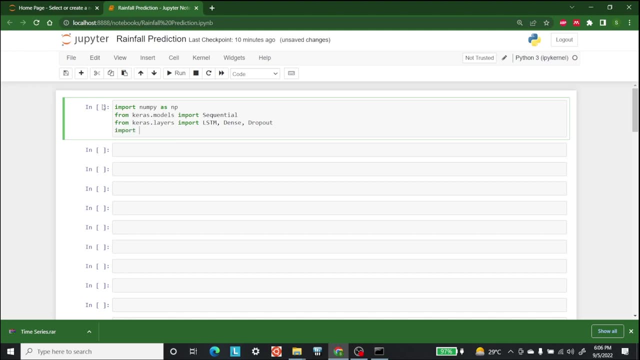 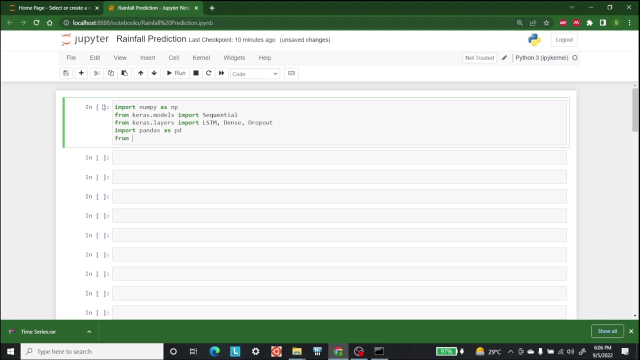 layers such as lstm, dense and dropout Right. So after that, the next step is to import pandas as pd, because we are going to use that. Other than that, we are going to use matplotlib, From matplotlib, import pyplot And at the end, we are going to use a scaling mechanism. 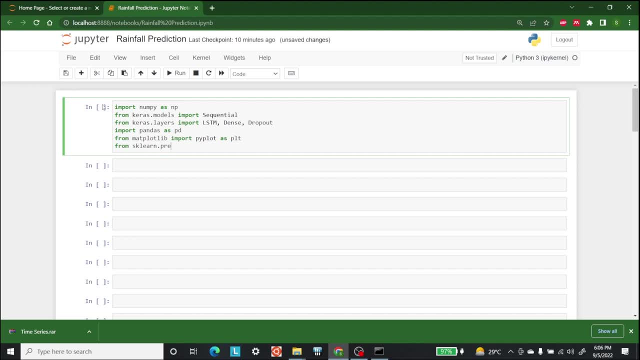 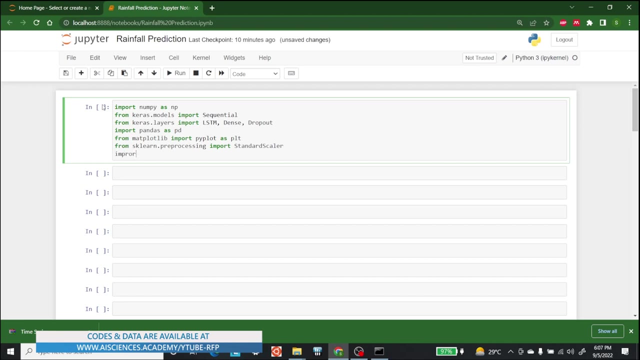 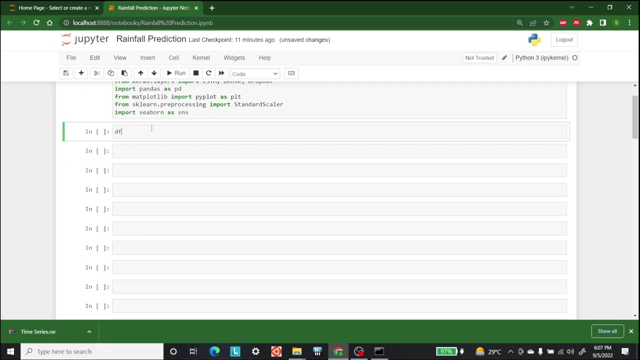 So let's write from sklearnpreprocessing import standard scaler And at the end let's import seaborn, Then import through pd And we're going to use it as a report. Let's record Debugger now. So let's create the report first. 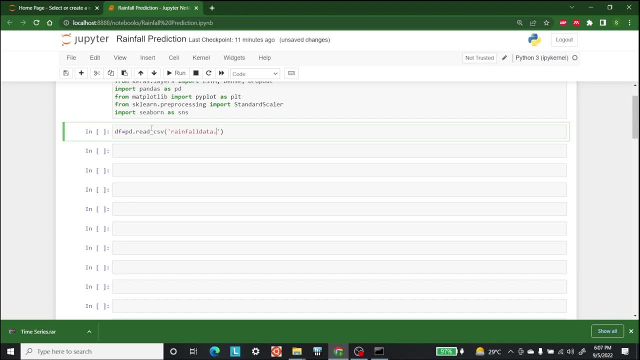 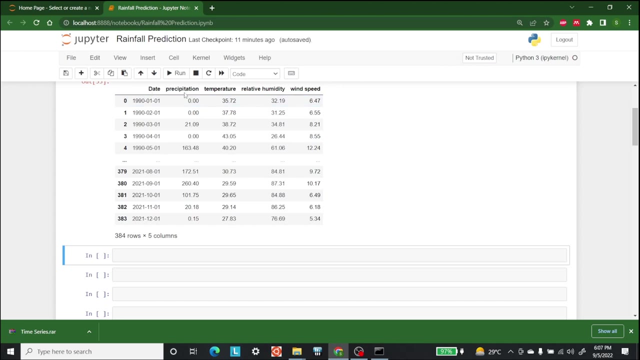 Now I'm going to edit it And then we're going to use憒 Set here dot csv. i have already saved that into my folder. now let me show you the data set. so this is the data set. it has one, two, three, four columns, and one column is for date. so the next. 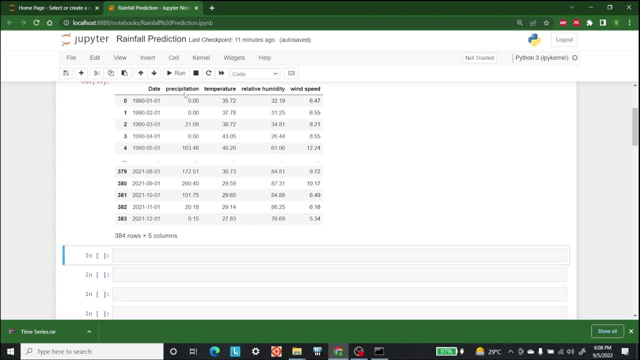 step here is to plot this data frame, to see how this is looking. so let's write df dot plot and let's write the kind of plot as line. other than that, let's give it a fixed size of 14 cross 8. so let's give it a title. 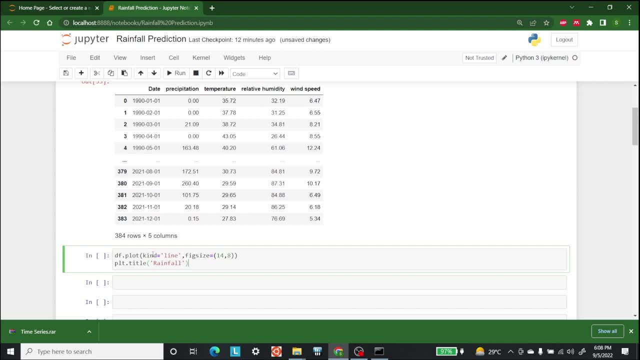 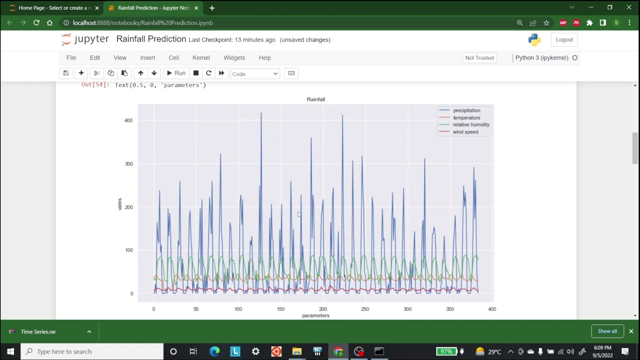 let's say the title is rainfall. after that, let's give it a y label, and the y label is values. and at the end let's give it an x label and let's say it has a parameters. so let's write parameters here. now this is the plot, as you can see. this is the precipitation. 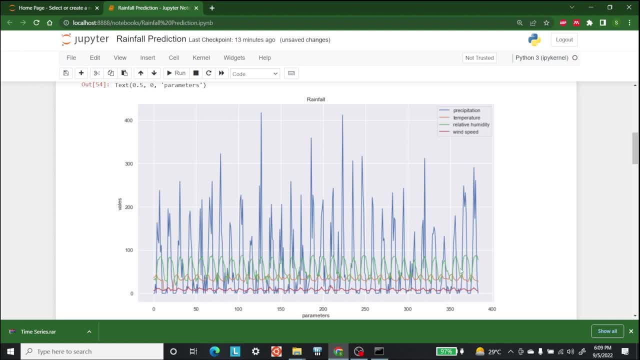 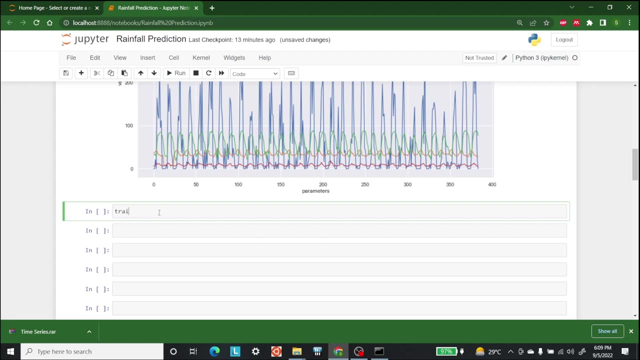 and here we have wind speed, temperature and relative humidity as well. so all of these things are plotted. now the next thing we are going to do is we are going to convert the dates and save them into train dates. so let's write: train underscore. dates is equal to pd dot two date time. that is the function. 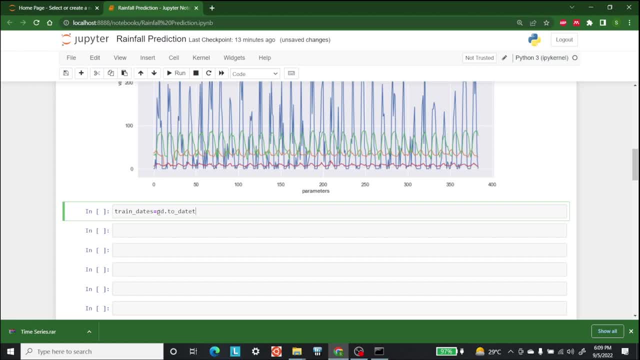 we are going to use to date time and we are going to enter the data frame into it and the column that we are going to use is date. let's run this and let me show you the data frame. let's run this and let me show you the train dates now. 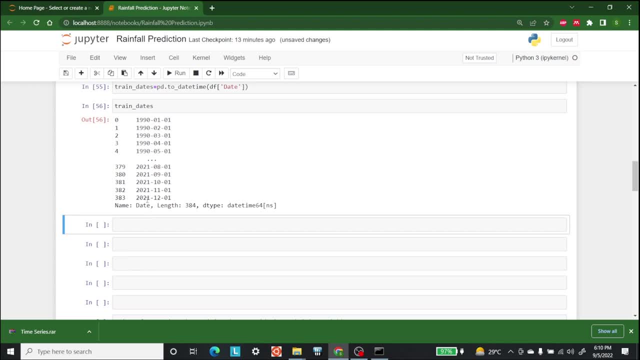 so these are the dates from 1990 to 2021, and after this we need to tell it which are the columns that we need. so the columns that we need is from first to fourth, right after the dates. so for that i'll write one to five. 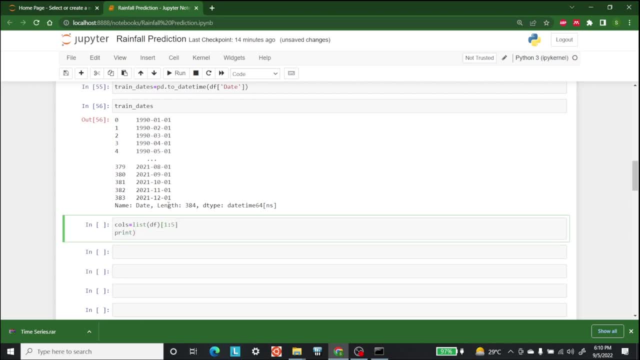 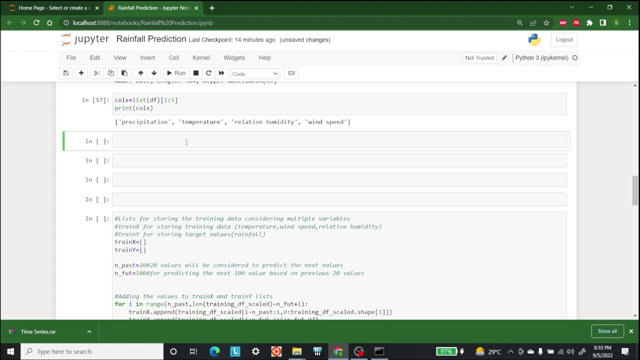 and then let's print columns. so there we go. these are the four columns that we have printed, and we can also know now, the column that we need from this is precipitation, which is the rainfall prediction column. so for that we'll write one column two, and this is the column that we needed. and now we have. 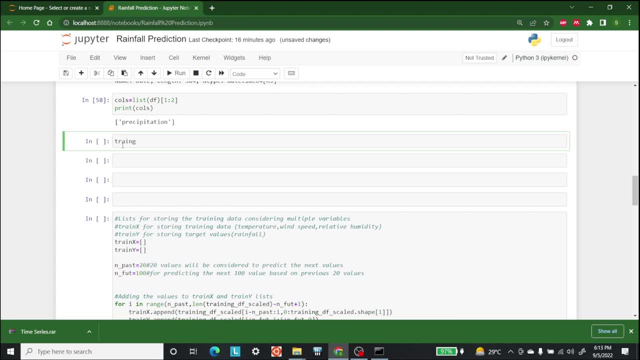 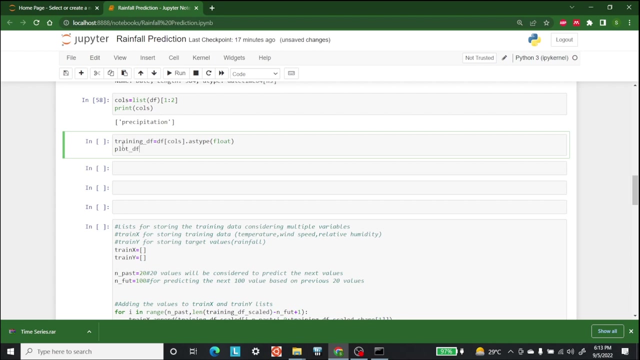 that now. after that, what we need to do is we will make our training data frame, which is equal to data frame, columns, dot as type and what is the type that we want? we want it to be float. after that, we can also show its plot by writing plot. df is equal to training df. 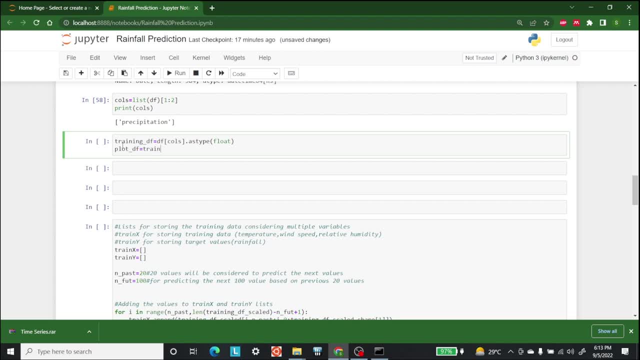 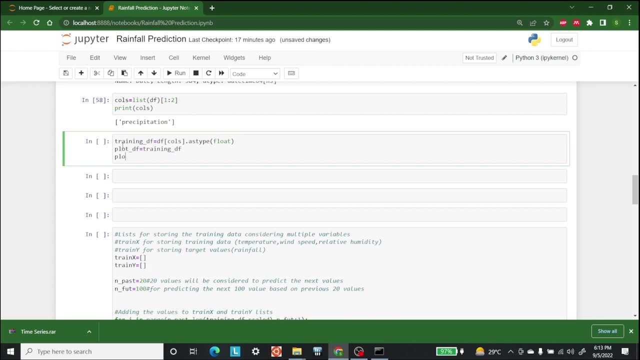 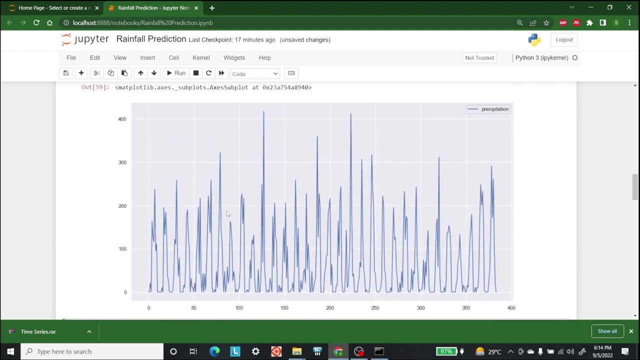 so after that we can just write training underscore df, and after this i can just plot it by writing plot underscore df, right and dot, plot, dot line. so it will show me the line plot. so there we go. this is the perception and this is its plotting. and now that it is saved in training data frame, let's start with this training data frame. let's. 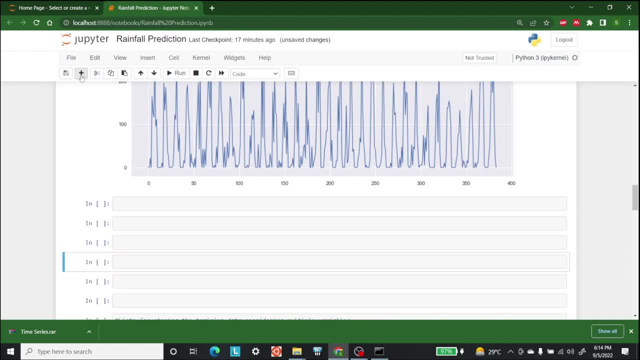 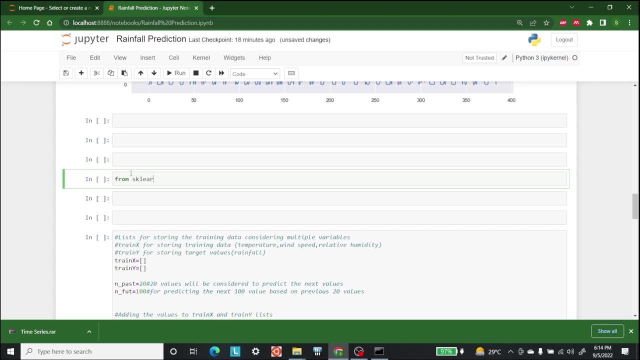 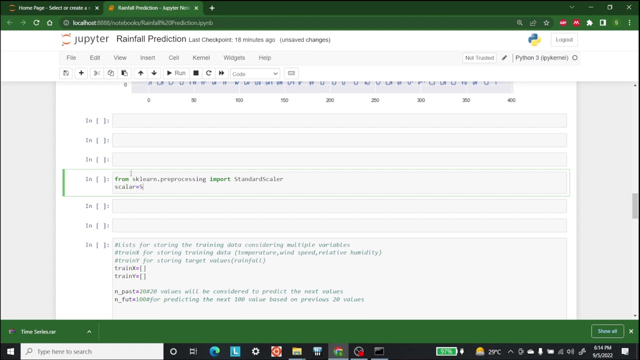 start with this training data frame, the scaling. so to perform the scaling, we need to write from sklearn dot preprocessing: import: standard scalar. after this, let's take a scalar. let's take a scalar and it should be equal to standard scalar right and after this, the next step. 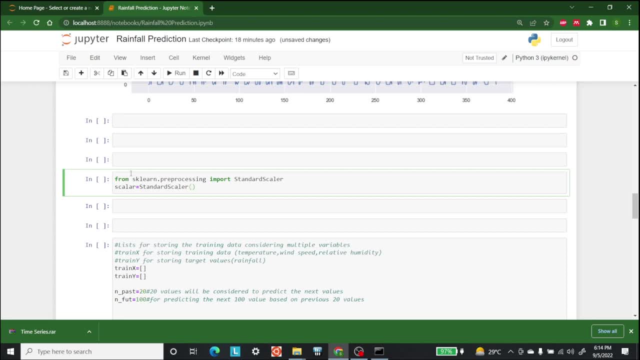 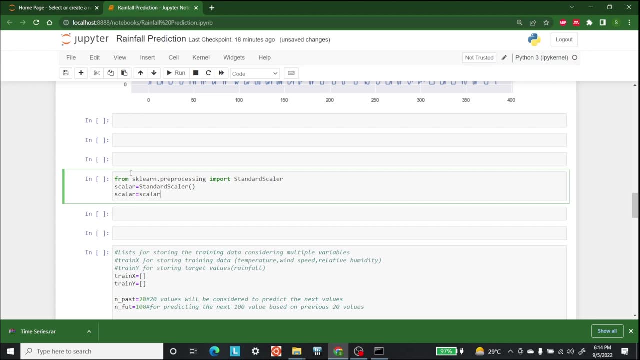 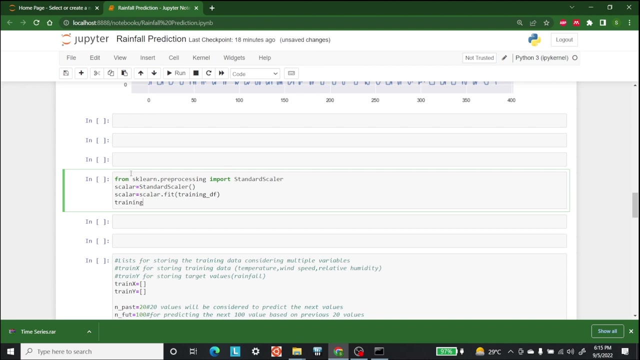 is to perform this, fitting on training underscore df, and at the end we are going to have a scalar that is equal to standard scalar, training underscore df, underscore scaled, and we are going to perform the scalar trans form and in this we are going to use the training underscore df. so let's do that. and now, 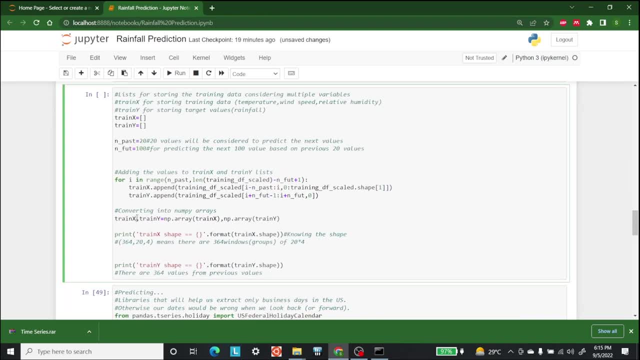 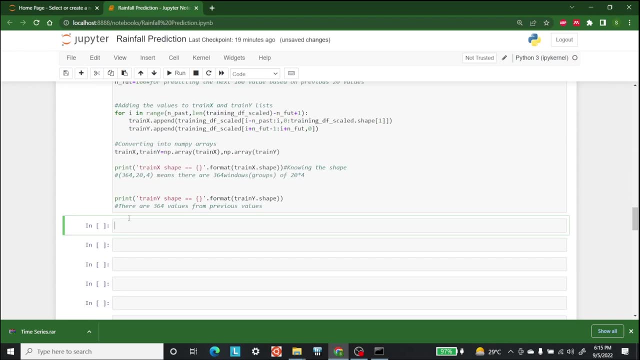 that we are done with scaling. the next step is to have a train x and train y values. for that i have also rec subconscious system-ämter algorithm stress- written a code. so now let's run that code as well. so there we go. this is the train x and train y shape. 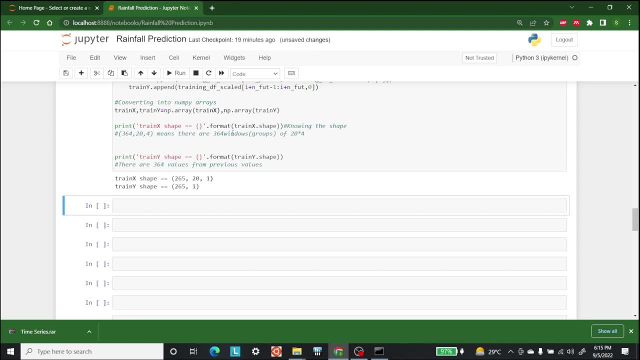 as you can see now, after this, the next step is computation of model. so the model is equal to sequential right. so for using the stacked lstm, we will first enter an lstm. lstm зависもしederailnonp negine between, we will first enter an. 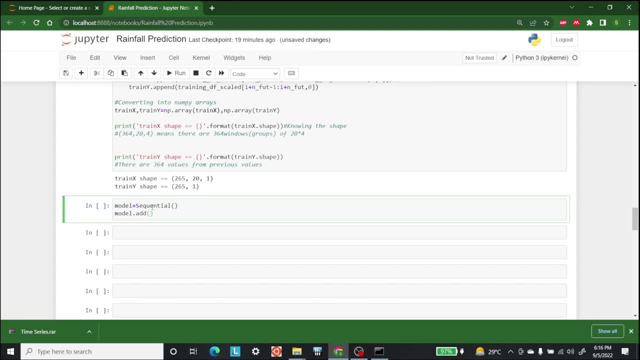 stm model for that let's say model dot, add, and then in lstm we are going to give it the neurons- neurons are 32. we are going to give it an activation function, so activation is relu. and after this we are going to give it an input shape, input, underscore shape and 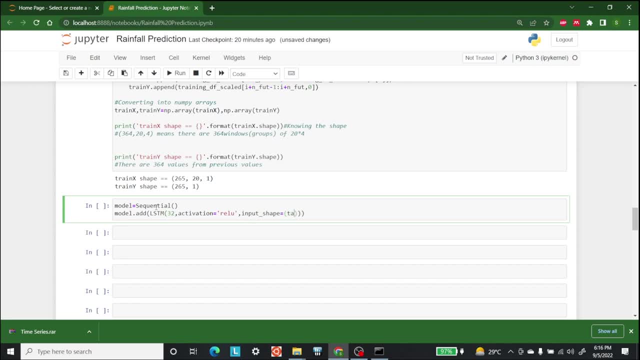 let's give the shape as train x dot shape 1 comma, train x- dot shape 2, and out of this we are going to write: return- underscore sequences is equal to true. so this is how you can add any lstm layer right. so after this, if we want more layers, 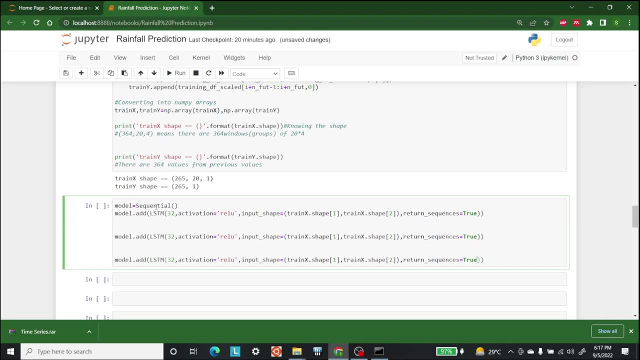 let's add three layers, so in this return sequences will be true also, but the input shape will be out coming from the previous layer. so we do not want input shape here, let's delete this. and we do not want ffiti input shape here. let's delete that as well. and here, because it is the last, 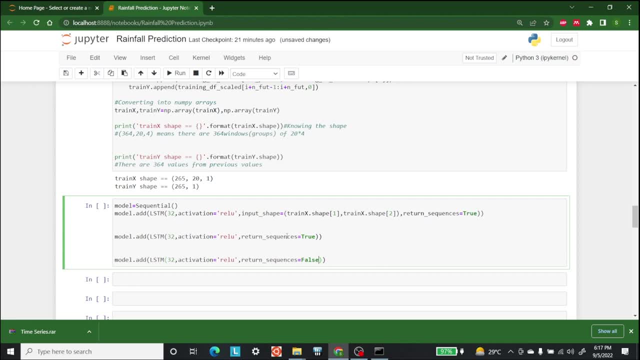 layer. we do not want a return sequence, so let's write false. after this, we need to add a dense layer for output, so for that let's write model dot add, and here I will write dense and what is the shape that I am going to use here I am going. 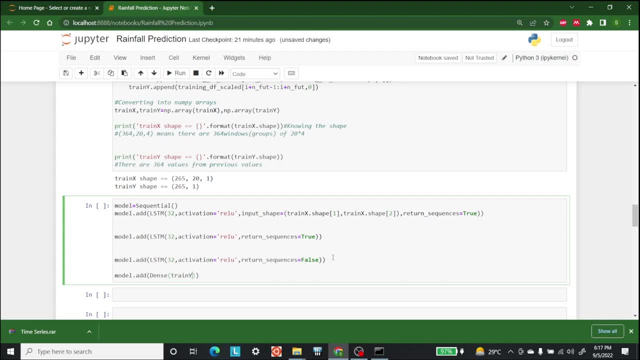 to use the train y shape. so let's write train y dot shape, right, so this is it. and after that we need to do the compilation. so for that let's write model dot, compile, and let's give it an optimizer, which is Adam, optimizer that we are going to use, and let's give it a loss, which is: 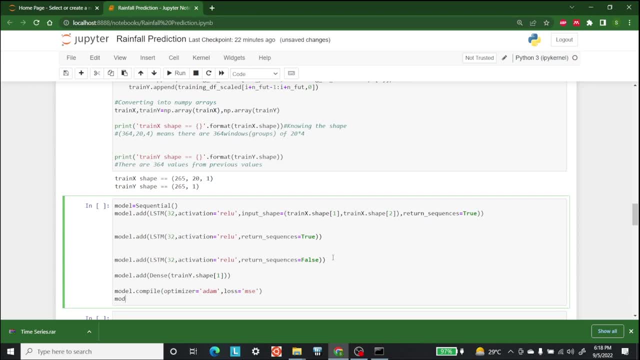 MSC, and at the end we are going to write model dot summary. now the last thing that we need here is we should add a few dropout layers as well. so let's write model dot add and so that it drops a few neurons if it's not working, fine. 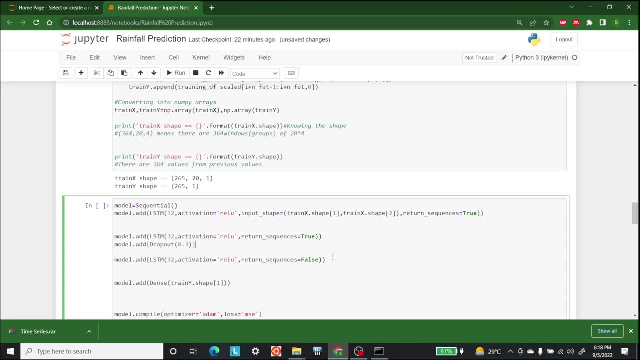 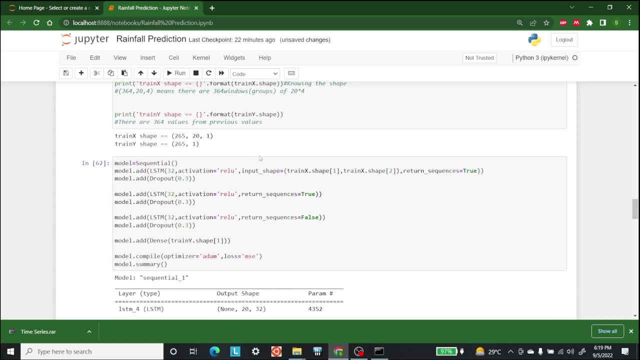 right, so let's write 0.3 here and let's copy this and let's paste it here, and let's paste it here, so dropout will be after each layer. so let's run this. okay, so we have an LSTM, then a dropout layer, then another LSTM. 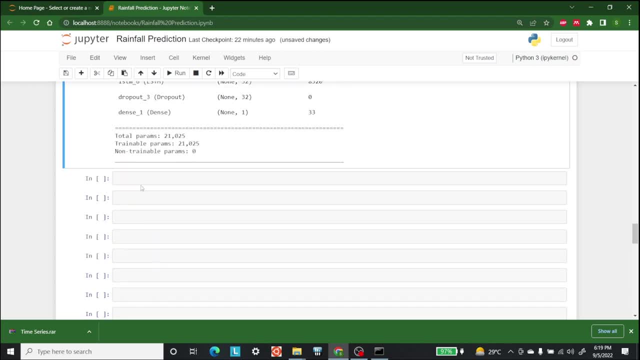 then a dropout layer, then another LSTM, then dropout layer and then a dense layer. so this is our model. after developing the model, we just need to fit it. so let's write: history is equal to model. dot fit right, and the connection of the wall doesn't need to be at the end, right, so we've. 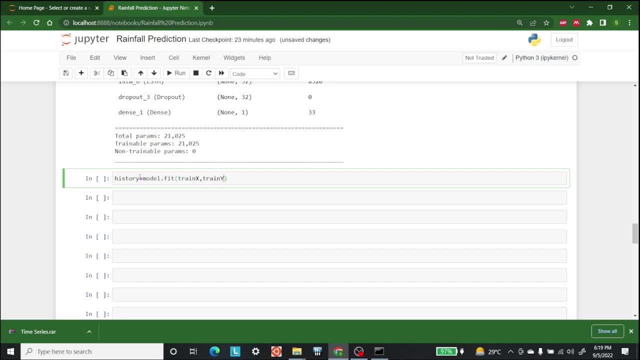 completed this and now the next step: we're going to give the next expression. so, as far as you know, it's not going to the end, right? so we're going to write zero and zero, and let's import your textbook as an example for equations as to the dot status, as we looked at this before you're going to head over to 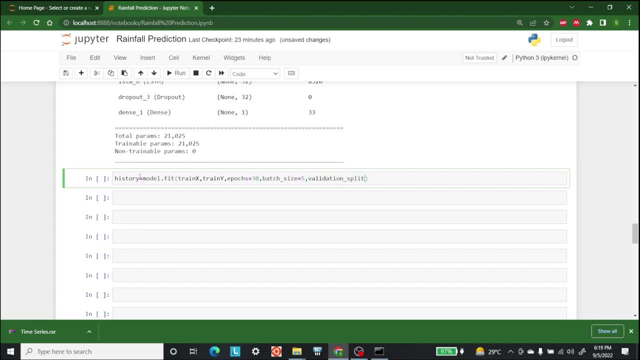 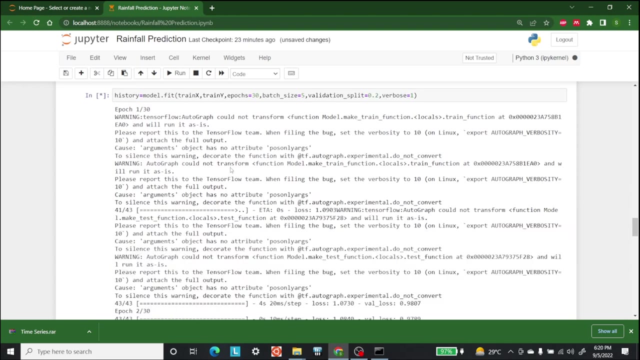 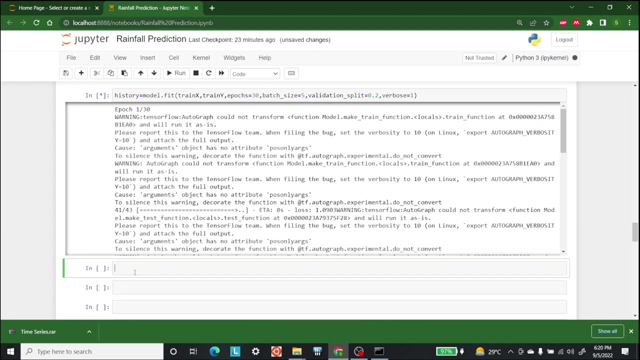 excel bye. and here we are going to write train X, Omar, plane white, and let's do it for 30 end. to see everything, let's write: verbose is equal to 1. okay, now that the training has been started, let us move on and plot this. so to plot it, we need to. 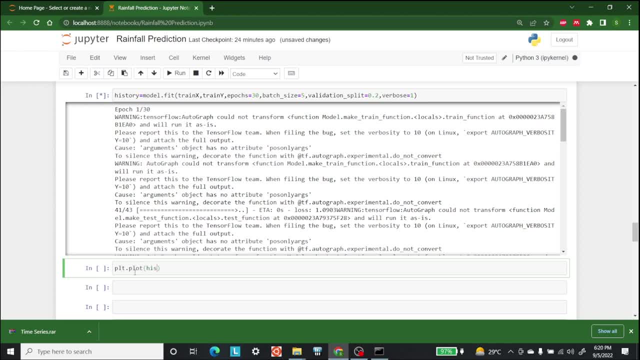 write PLT dot plot. and here we will plot two things. first thing is the validation loss and second thing is the training loss. so for the training loss we just have to plot loss, and here we will give it a label. so label is equal to training loss, and in the same way we will also.